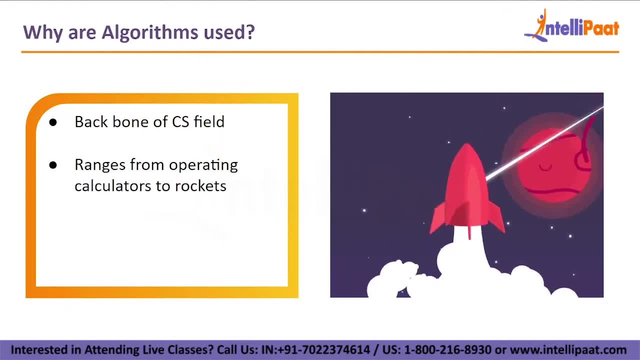 instructions that allows a computer to perform any tasks, such as operating a calculator or launching a rocket, for instance. algorithms are used by Google engineers to improve searches, forecast what users will enter and more. knowing how to create an algorithm is an important component of a computer program when it comes to problem solving. now let's move on to our next topic. 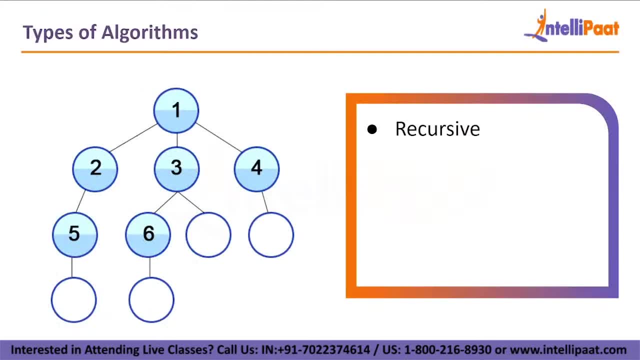 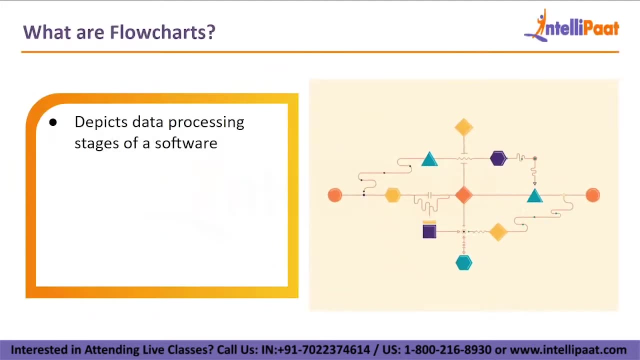 types of algorithms. essentially, there are six different types of algorithms that are most commonly used. they are recursive, divide-and-conquer, dynamic programming, greedy brute-force and backtracking. now let's go to our next topic: what are flow charts? a flow chart is a diagram that depicts the stages of a software or an 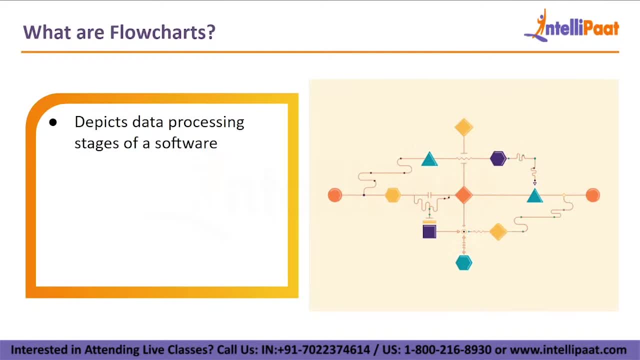 application that takes to process data. several geometric patterns can be used to show the different tasks that the software or application does. the designer may efficiently separate the various aspects of the process using flowchart. it also makes the analysis easier by providing step-by-step directions on how to solve the problem. 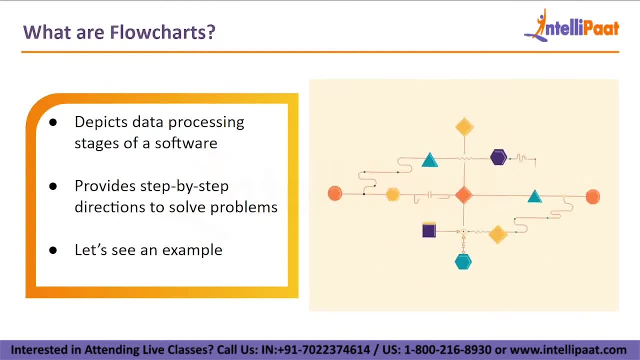 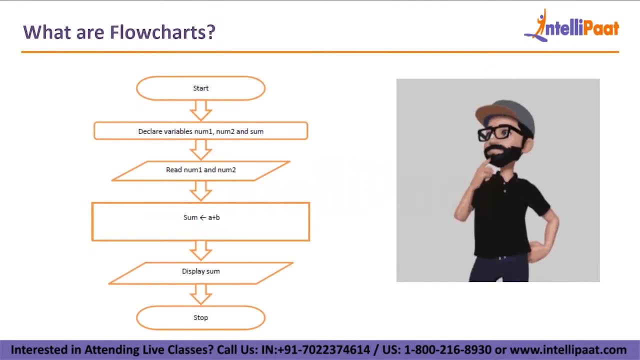 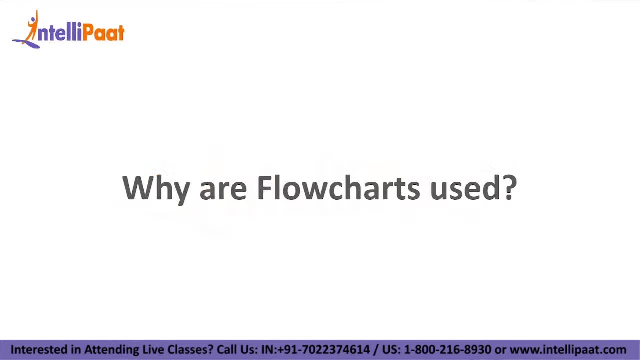 let's see the example for the same problem of adding two numbers that we took for the algorithm example earlier on. yeah, it starts, and then you can see that we are using various symbols and shapes in order to depict different types of actions. now let's get to our next topic, which is why our flow charts. 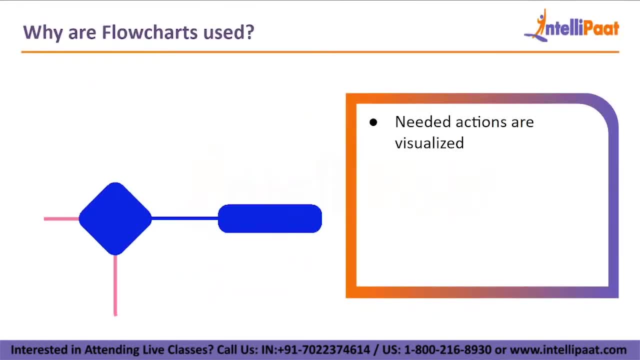 used any flow charts. objective is to aid a location走吧 INTO the target of a preference. we are making an area specific to the specific field of the information that the process requires for a particular project. process is updated, often in the form of�� fahrni. 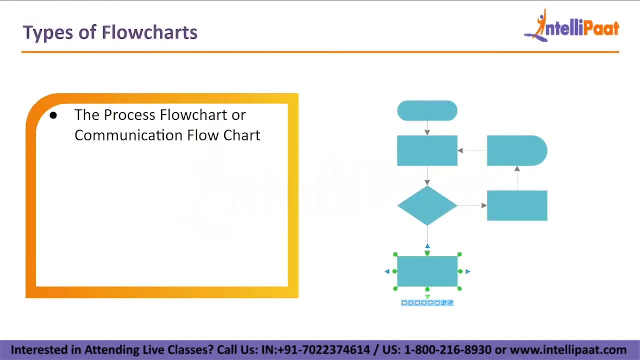 you hear a beautiful, slow, clear me. use flow charts. if you think you'd be interested in learning about the flowcharts, present is under heavens and fade, or the communication flowchart, the workflow chart or the workflow diagram, the swim lane flowchart and finally, the data flowchart. Okay, so let's see what our next topic is. What are pseudocodes? 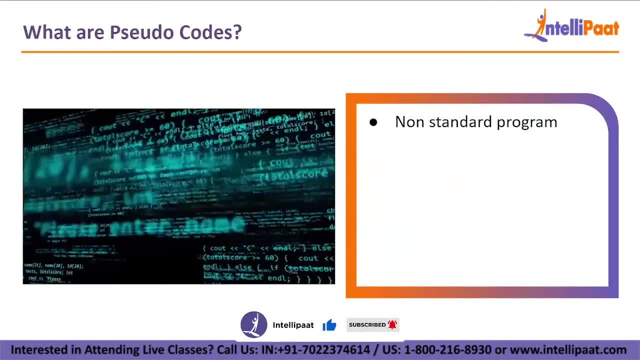 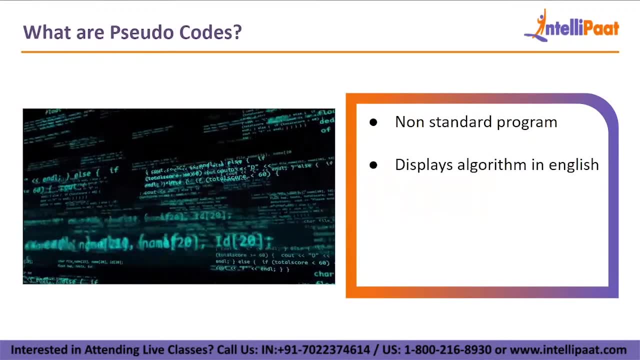 A pseudocode is a slang term for a non-standard manner of writing a program. It is not, however, a computer program. It solely displays the program's algorithm in a normal language and mathematical notation. Furthermore, there is no specific programming language for creating. 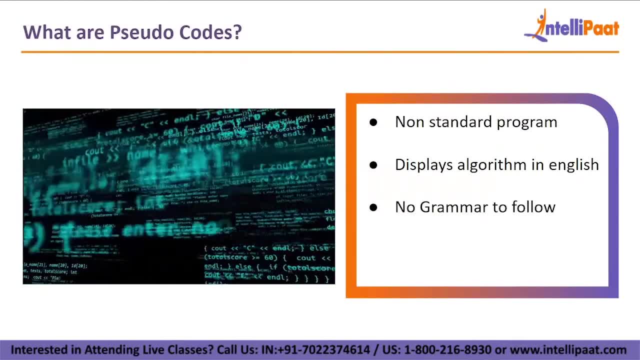 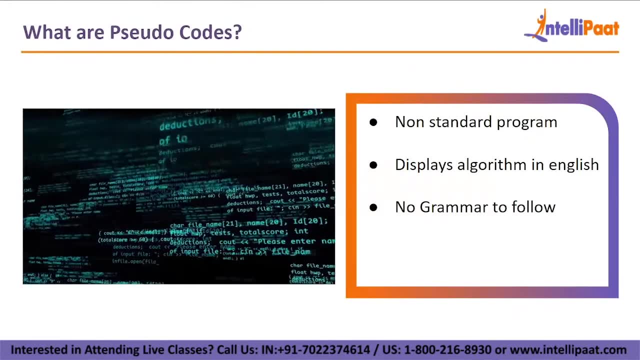 pseudocode. When developing pseudocode, there is no grammar to follow, unlike in real programming languages. Furthermore, basic English language expressions can be used to create pseudocodes. Hence it is something that lies in between a fully fledged, syntactically correct code. 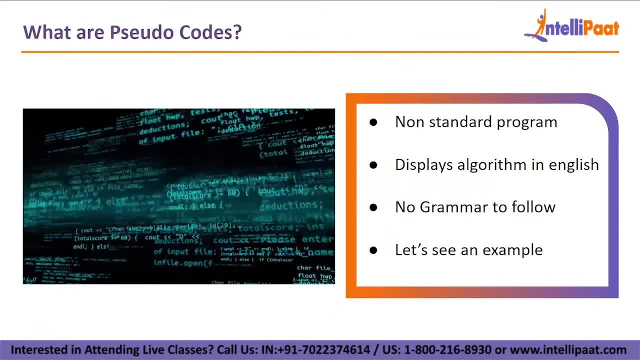 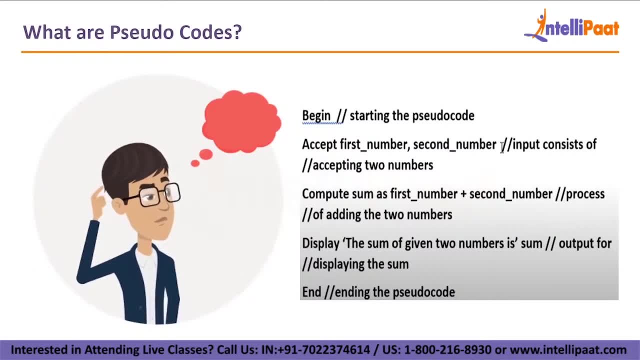 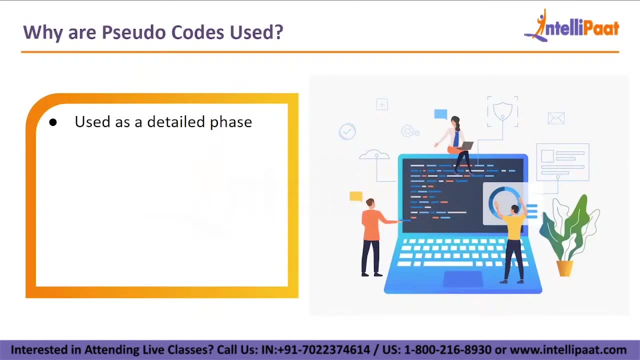 and a well-formed, grammatically correct sentence that describes the algorithm and working of the program. Let's see the example for the same adding of two numbers. Now let's get to our next topic, which is why are pseudocodes used? Pseudocodes is occasionally used as a detailed phase in the development of a program. 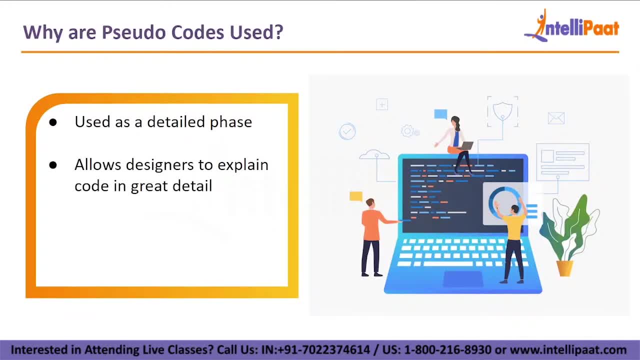 It allows designers or lead programmers to explain the concept in great detail and give programmers a thorough template for developing code in a specific programming language in the following stages. Because pseudocode is comprehensive but accessible, it may be examined by a team of designers and programmers to confirm that real programming 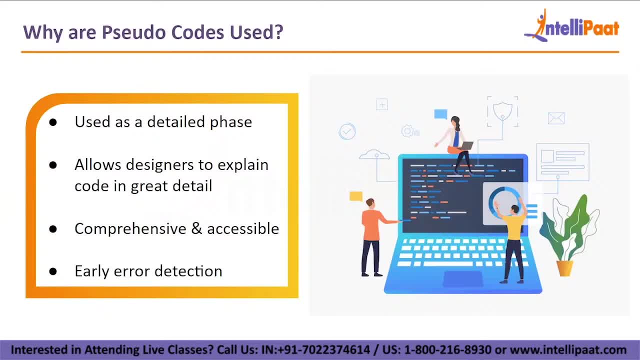 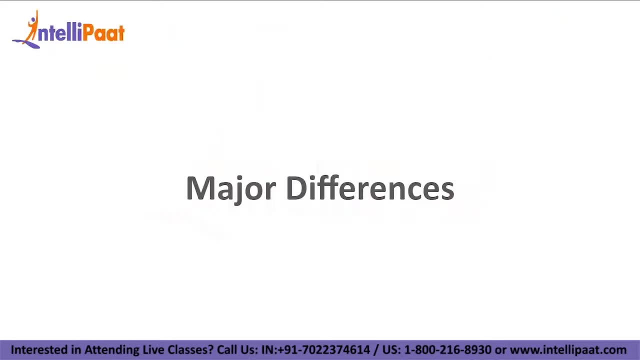 matches design criteria. Catching problems early in development process is less expensive than catching them later. Once the pseudocode is accepted, it is rewritten using the vocabulary and syntax of a programming language. Now let's move on to our final topic of this session, which is major differences. 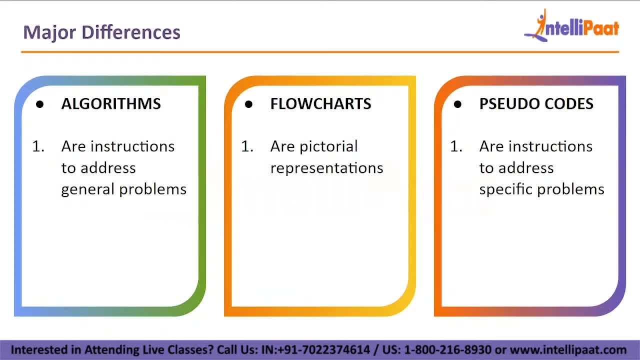 Algorithms are instructions to address general problems. Flowcharts are pictorial representations. Pseudocodes are instructions to address specific problems. Algorithms are written in pure English and mathematical notations, with no general writing rules. Flowcharts are represented by symbols and shapes. Pseudocodes are written in English. 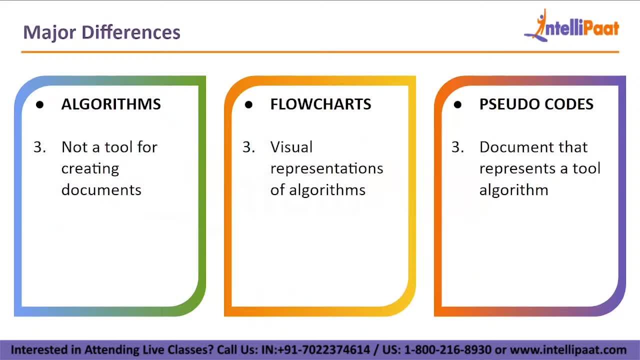 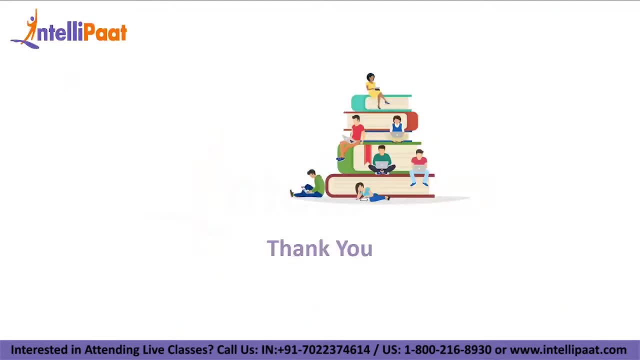 but they do follow a set of rules. Finally, algorithms are not tools for creating documents. whereas flowcharts are visual representations of the algorithms that are already created, Pseudocodes are documents that represent a tool of algorithms. That's all for this video. Thanks for watching. Make sure you're subscribing to our YouTube. 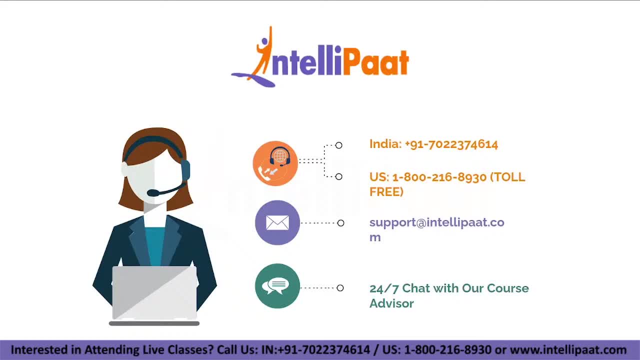 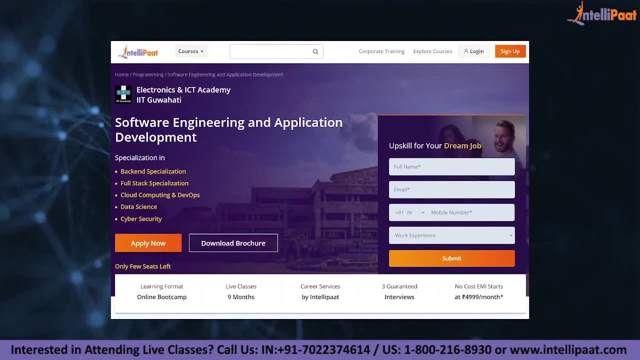 channel and enabling that bell icon so that you'll get all the updates from Intellipaat regular. Just a quick info, guys. If you want to make a career in software engineering, then Intellipaat provides an advanced certification program on software engineering and application.